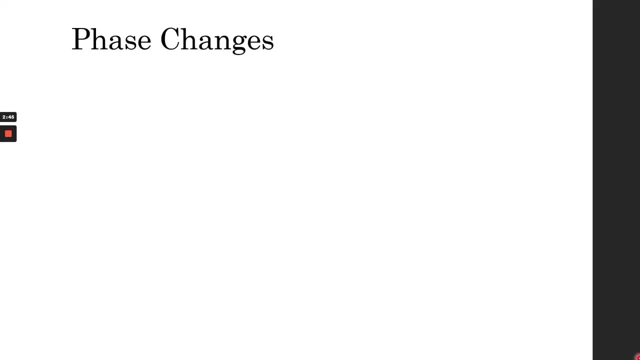 water and carbon dioxide. First let's discuss what are, or what is phase change. Phase changes is when matter changes from one state to another, and there are six phases of phase changes, and they happen whether temperature decreases or when it increases. Also, atmospheric pressure is related to it, but for intents and purposes for now, let's say that the attribute 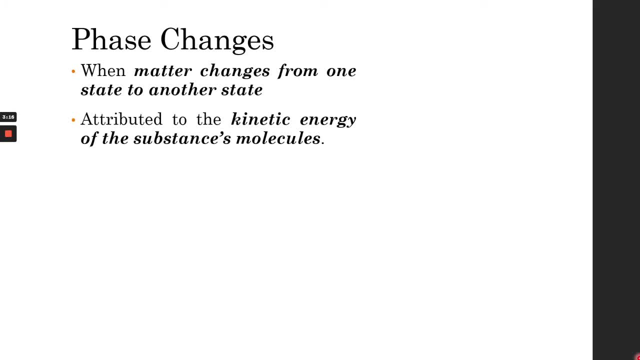 the phase changes is attributed to the kinetic energy of the substance's molecule. So the phase changes are related to the kinetic energy of the substance's molecule. So there are six phase changes of matter. When temperature rises, melting happens. that's when- when solid matter turns to liquid. Also, sublimation can happen. that's that is when solid turns to gas. 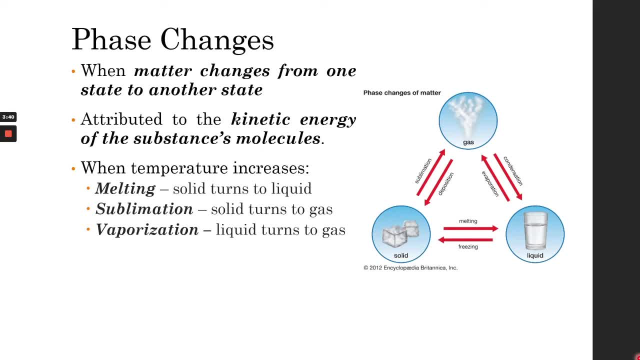 The other one is called vaporization, that is when liquid turns to gas. When temperature decreases, another phase changes, phase change happens. One is called vaporization, condensation, which when gas turns to liquid. the other one is called freezing, which when liquid turns to solid, and deposition, when gas turns to solid. so melting is when liquid turns to. 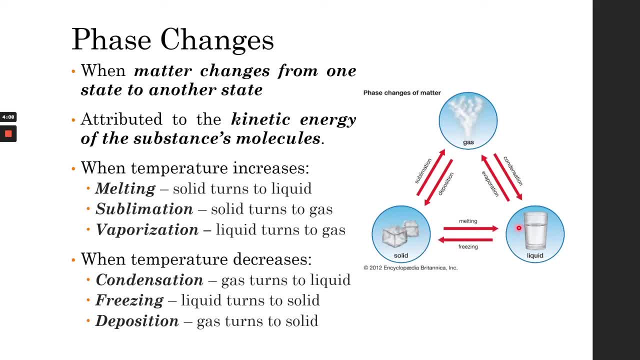 or when solid turns to liquid that's melting. sublimation is when solid turns to gas, and vaporization or evaporation is when liquid turns to gas. condensation is when gas turns to liquid. freezing is when liquid turns to solid and deposition is when gas turns to solid. 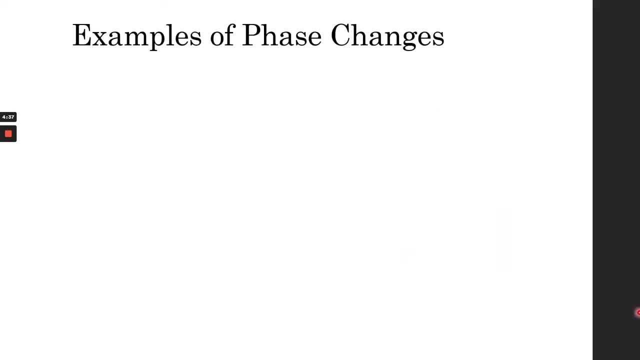 so some examples of phase changes that are present in the world. one is melting. the most clearest example is, of course, ice, which is solid water, and change to liquid water. but another thing that is an example of melting is lava. lava is basically molten rocks. sublimation in the example is dry ice. 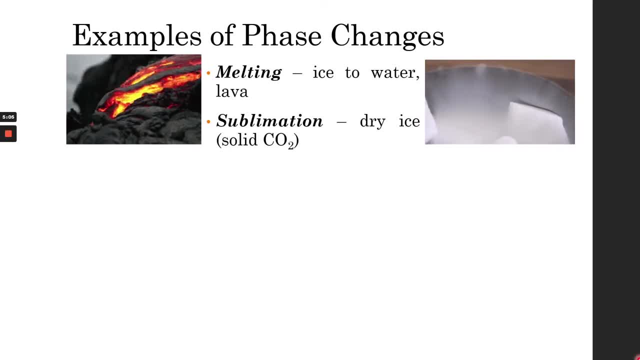 so dry ice is actually a frozen or solid co2. so when you have solid co2, as you can see in this moving picture right here, you can see kind of like the mist that is escaping the solid. so that is a sublimation wherein the solid, dry, solid co2 changes its phase. 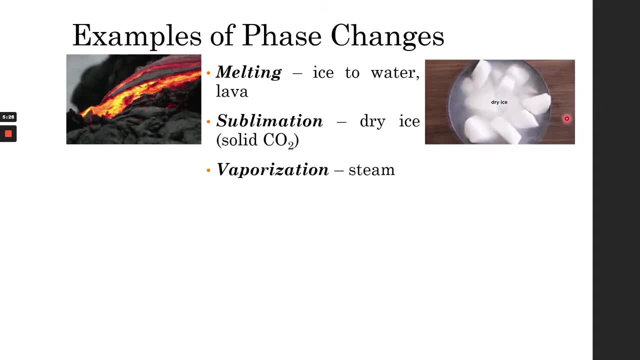 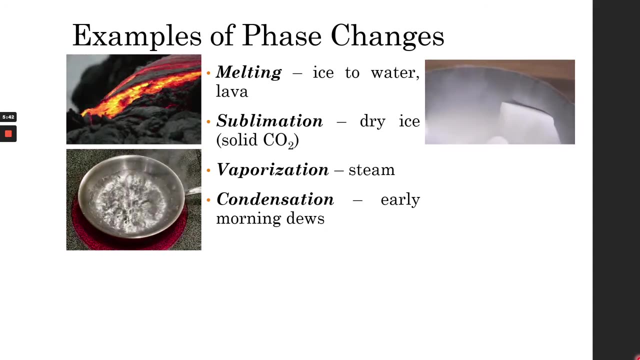 from solid to gas. another one is called vaporization. the clearest example is, of course, is steam, when we are boiling water. next one is condensation, that is, when gas turns to liquid. one of the best example of condensation are the morning dews, wherein if you guys wake up early in the morning and go outside and check out, check on. 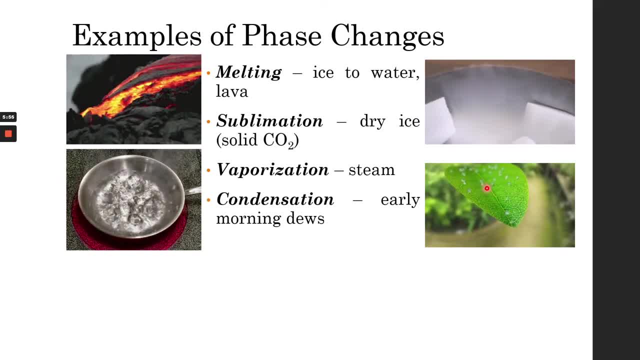 some leaves and branches. sometimes you would see droplets of water on the grass or on the leaves, even though it didn't rain last night. so those are actually condensation we're in because the temperature decreases at night. the, the, the water vapor or the gas water present in air changes back from gas to liquid, so those that's. 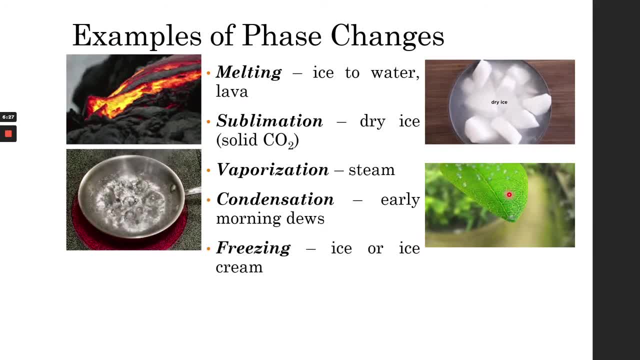 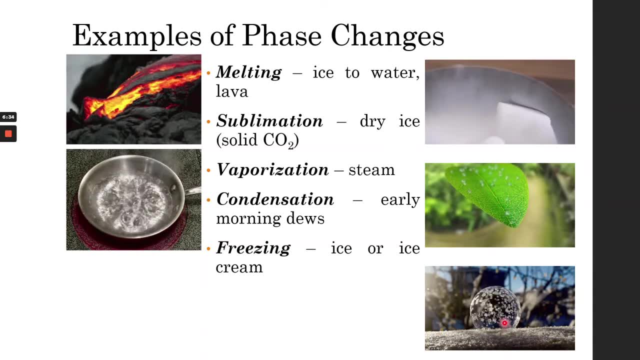 what you see the dews in the early morning. next one is freezing. the most common thing is, of course, ice or ice cream. here's an example of a. we have a water with its water particle around the bubble and it freezes. so when we have water particles, that freezes. 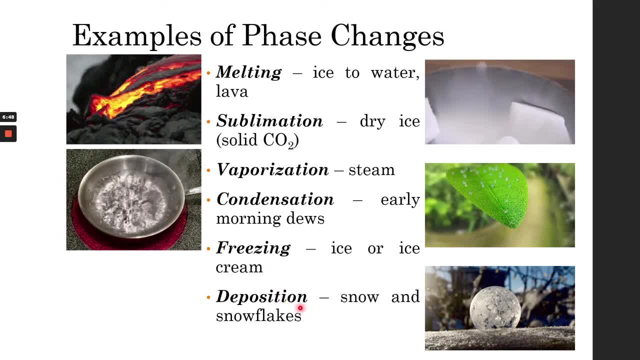 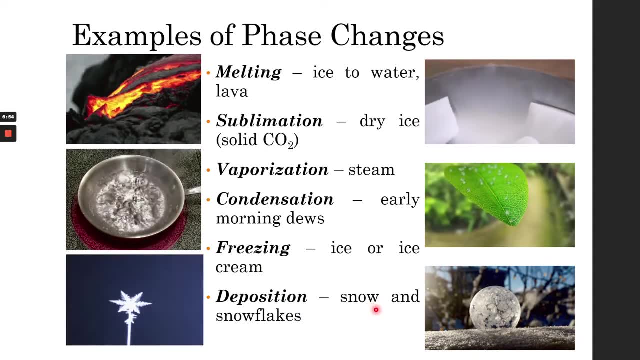 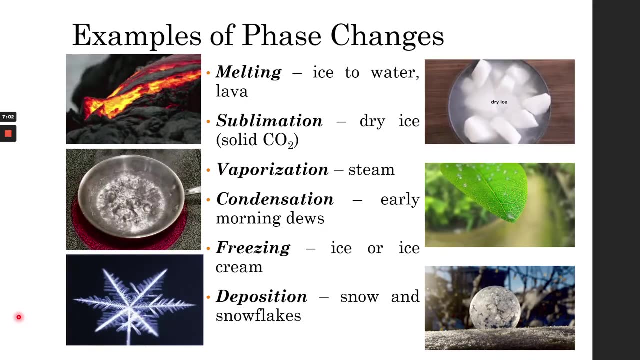 liquid that freezes. that's freezing. deposition is when gas turns to solid. one of the best examples is snow and snowflake. so snowflakes is actually when the gas, because it's too cold, it changes immediately from liquid vapor, which is our water gas, to a solid water. as an example is a snowflake. 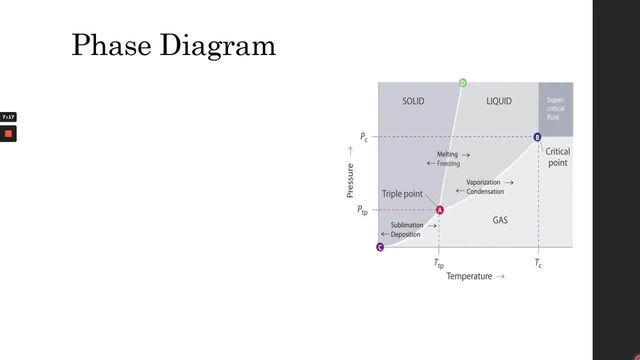 right here. so what is the phase diagram? so phase diagram is basically a graphical representation of the relationship between pressure, which is is on the y-axis, and temperature, and how pressure and temperature affects the three phases of matter. in phase diagram you would see three areas where there is solid, there's liquid area and there's gas. and depending on 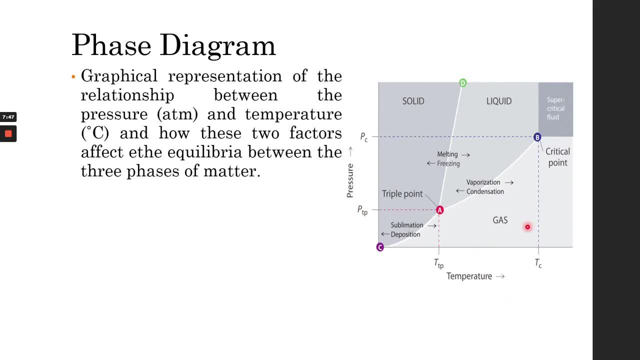 the pressure and temperature a substance phase can change and the phase diagrams basically tells you what pressure it needs, at what temperature for one uh substance to change its phase from either liquid to solid or vice versa, or from gas to salt to liquid and vice versa, or even solid to 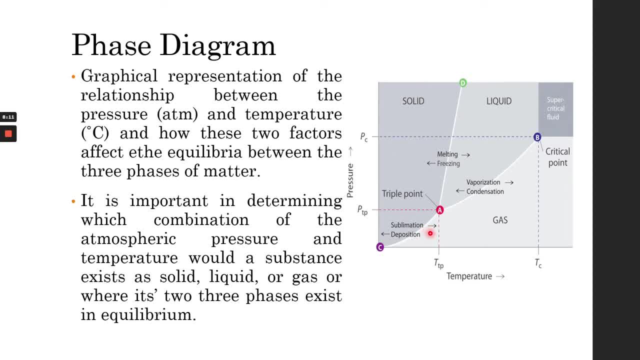 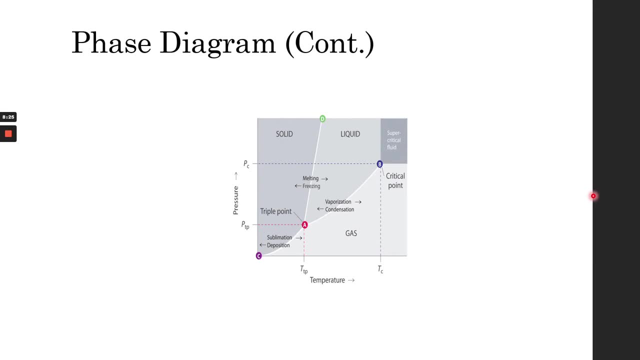 gas and this is important in determining, like i said, the combination of both the hot and the cold, of atmospheric pressure and temperature, to determine what combination we need to change for phase changes. So a phase diagram includes what we call a fusion curve. So if you have a picture, let's just look at the picture right here. So we have. 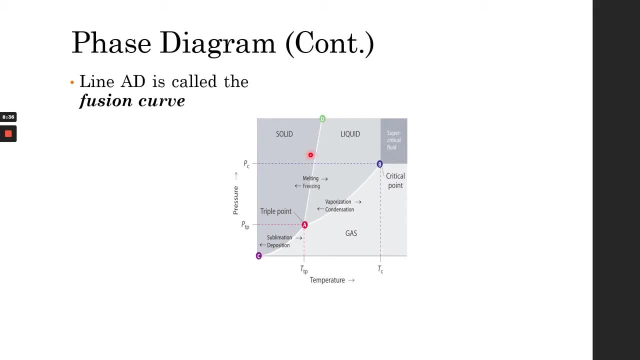 point A and you have point B. So this line between point A and point B is called the fusion curve, or the curve or the line which separates the solid from liquid state of a substance. But also in between this line the solid and the liquid phase of that substance is at equilibrium, So it's equal parts solid. 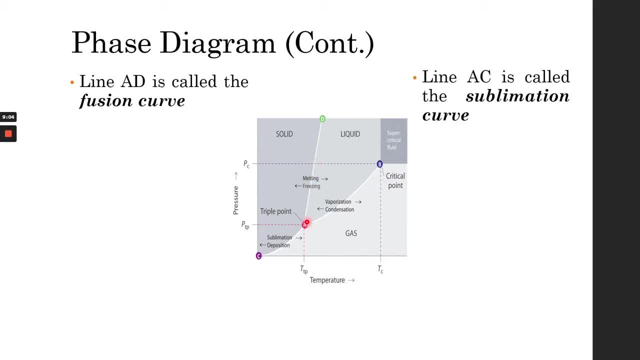 and equal parts liquid, So the A-Z line. so this A-Z line is the line where there will be liquid and there will be a solution. This line does not have the equilibrium part of this series. Now that this line here will have the equilibrium parcel by E and theрbih islands, so that they will not have the equilibrium. Now she starts from where to 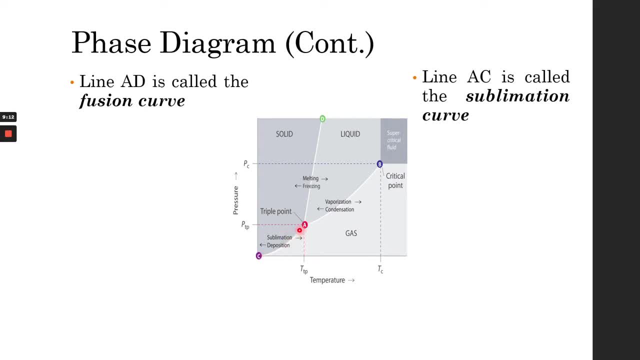 right here is called the sublimation curve, so it's the curve that separates the solid from gas, and this curve right here is the uh, the characteristic of the substance. substance on this line right here is when solid and gas is at the equilibrium. the third line is called or uh. 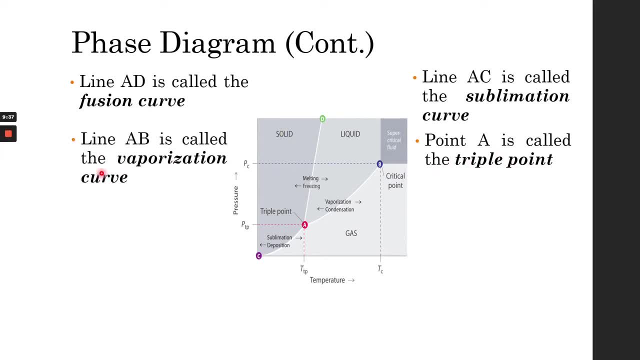 oh, there's another line that's in here. so the third line from a to b is what we call the vaporization curve. this is the line that determines or that separates the solid and the gas. so there's a point right here. uh, this point a right here is called the triple point. 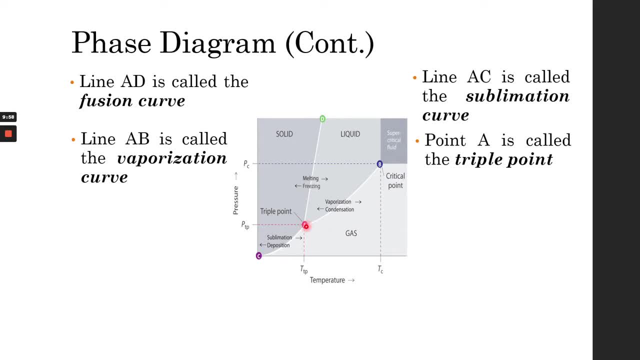 this is where the characteristic of the substance we're in its solid phase, its gas phase and its liquid phase at it is at its equilibrium. so, basically, this is the point where the solid liquid and the gas phase of one substance or matter is at equilibrium. so they're. 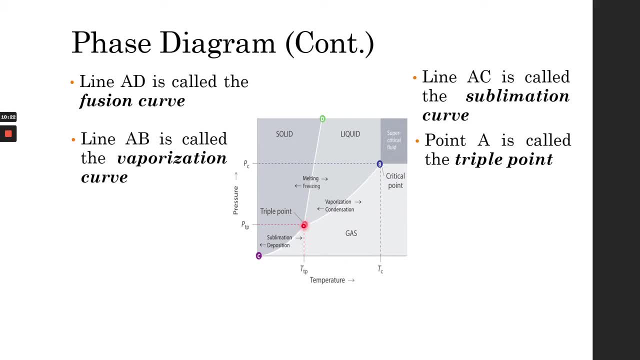 all equal solids, equal liquid and equal gas. so it's continually changing from solid to liquid, to gas. so it's at the equilibrium at this point. another point is called the critical point. so the critical point is called the critical point and the critical point is called the critical point. 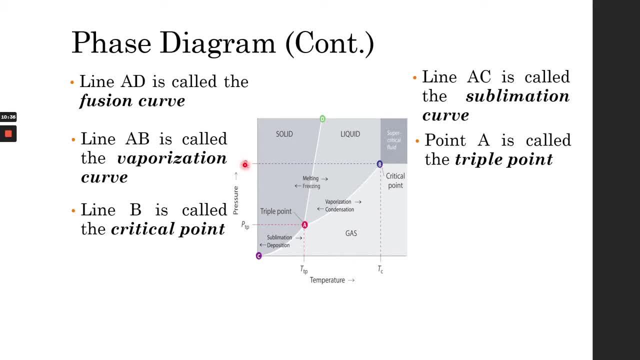 point is where, when a substance reaches a certain pressure, at a certain temperature, it is impossible to distinguish whether it's liquid or gas. when that happens, the liquid is called, or the substance is now and it's is called a supercritical fluid, wherein you don't know, or. 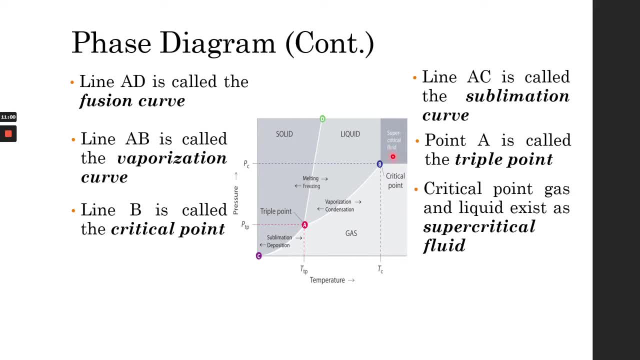 it's indistinguishable whether the phase of that matter is liquid or gas. again, there's three areas that separates the phase diagram: the solid, the liquid and the gas and the pressure. it's a y-axis and the temperature is usually at the x-axis. so now let's look at the phase. 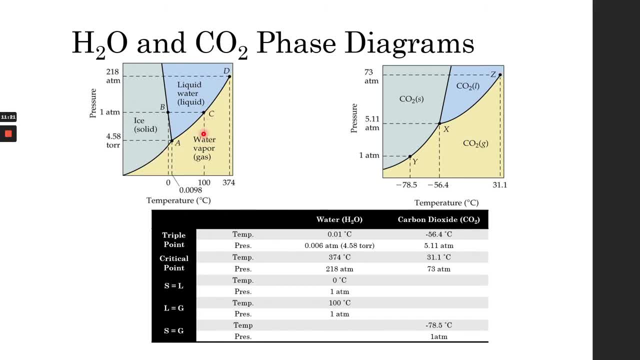 diagrams of water. so this picture right here at the left is the phase diagram of water and the picture right here is the phase diagram of co2 or carbon dioxide. so i tabulated the temperature and the pressure for water and carbon dioxide. so at the triple point, if you guys remember, this is the point where all 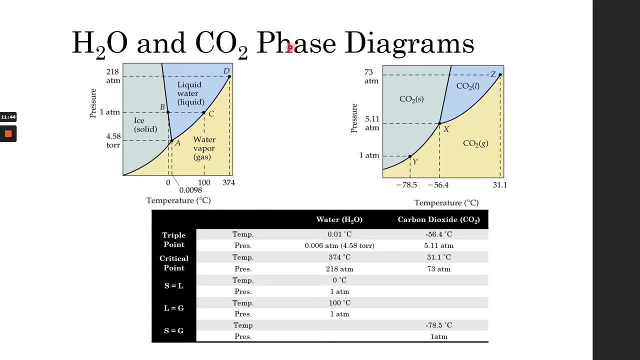 the phases of, in this case water and carbon dioxide, is at equilibrium. so the temperature for and the pressure for the triple point for water is at 0.01 right here. 0.01 or 0.0098 degree celsius, at 4.58, or basically 0.006 atmosphere. that is the point where the water 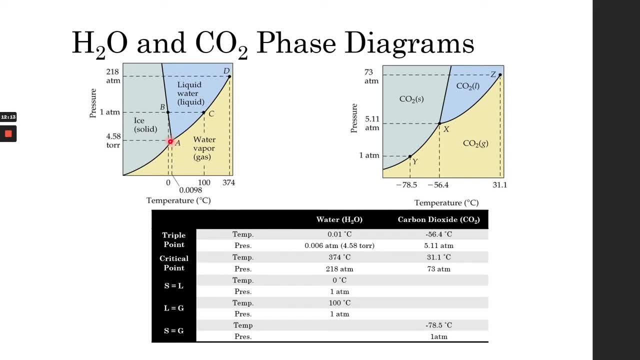 solid, liquid and gas phases are at equilibrium. for carbon dioxide it is at negative 50- 6.4 degrees celsius, with an atmosphere of 5.11. so the critical point: where is the point where you cannot distinguish between the solid and the gas phase of that matter? for water it's at 374 degrees celsius and a 218 atmosphere. so this: 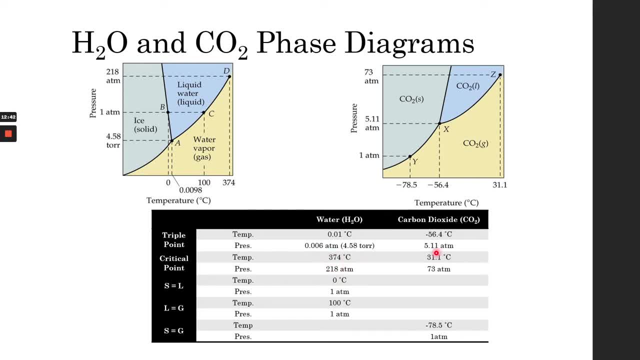 is very high pressure and very high temperature. the same situation for the critical point of carbon dioxide: at very high temperature and sort of a relatively high atmosphere that the supercritical fluid of carbon dioxide exists. so the curve, or in the solid, in the liquid phase of water. 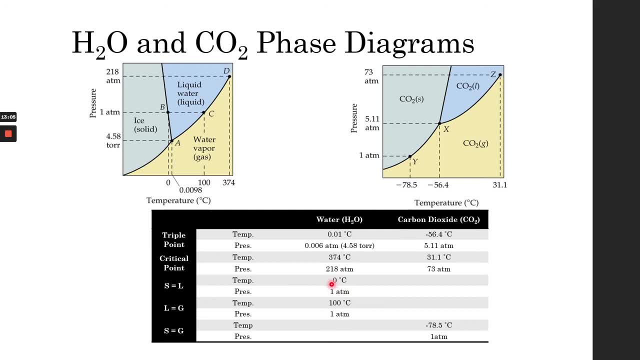 is almost equal, is at zero degrees celsius in one atmosphere. so meaning the water liquid, the liquid water turns to solid and also it's going back and forth. so lowering the temperature would cause us to this point, right here, at one atmosphere, at zero degrees celsius. 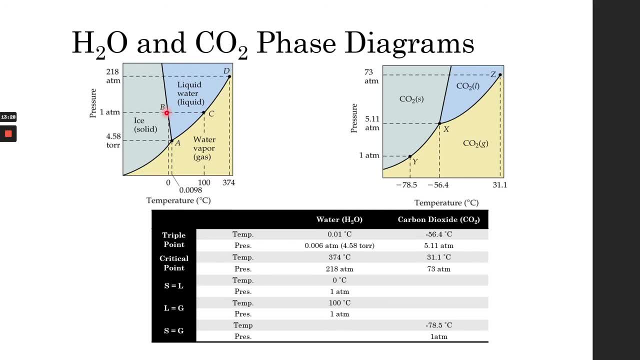 point b right here. so water is at an equilibrium in its solid and solid and liquid state. so lowering temperature would cause the water to freeze and increasing the temperature to make it water. so i just tabulated: for carbon dioxide it doesn't have. it doesn't have also where the liquid and the gas is. 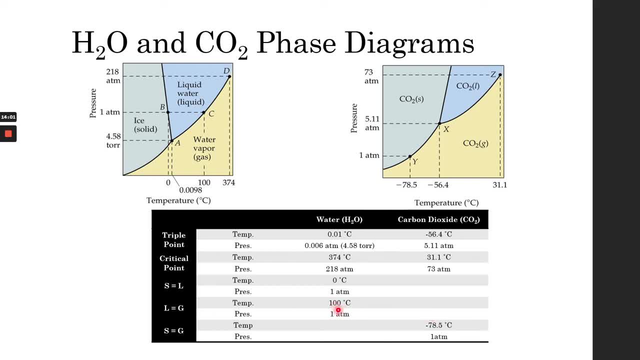 at equilibrium. but for uh water- 800 degrees celsius at one atmosphere- the water boils where the water is equal towards to gas. but for carbon dioxide we can solidify it and at the same time it's gas. if you guys remember, solid carbon dioxide is basically dry ice, so you can create dry ice at 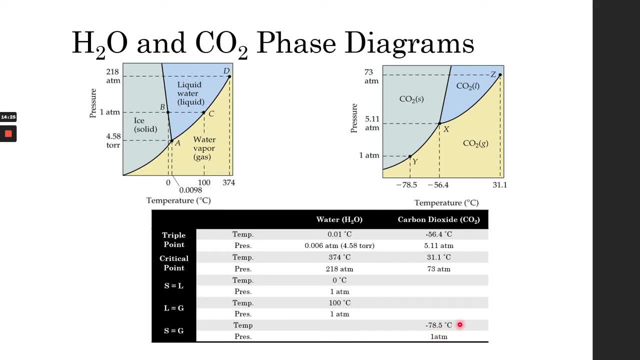 negative 75- 78.5 degrees celsius. it's really really cold at one atmosphere. so you can- actually it's possible to create solid carbon dioxide, but in normal situations you can't, because that's this is too cold for humans to survive for long periods of time. 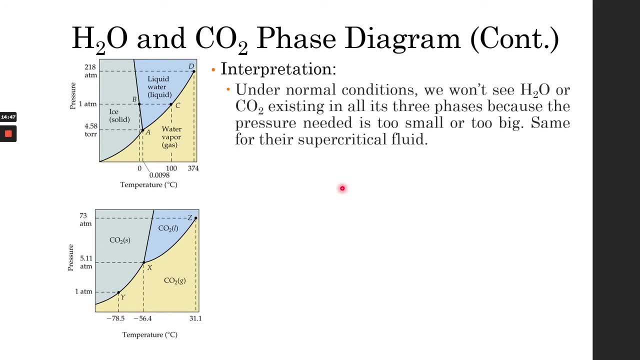 okay. so how do we interpret this phase diagram under normal conditions and it's difficult to see water and carbon dioxide existing in all its three phases, so many at certain. a normal condition is difficult to see the water and the carbon dioxide when they are a triple point. this is: 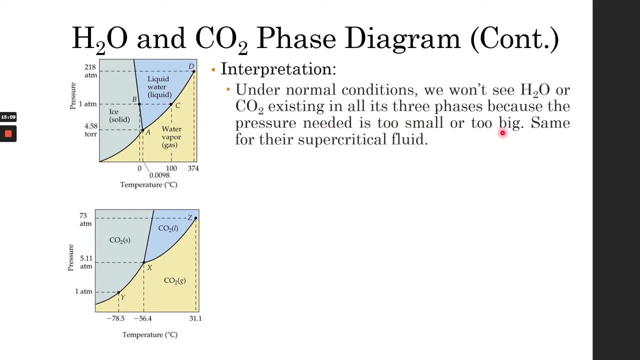 because the pressure needed is too small or too big at the same time. it's the same situation for conditions. so unless you create them in a laboratory setting, you cannot see a super critical fluid water or super critical fluid co2 at the same time, also when they're existing in. 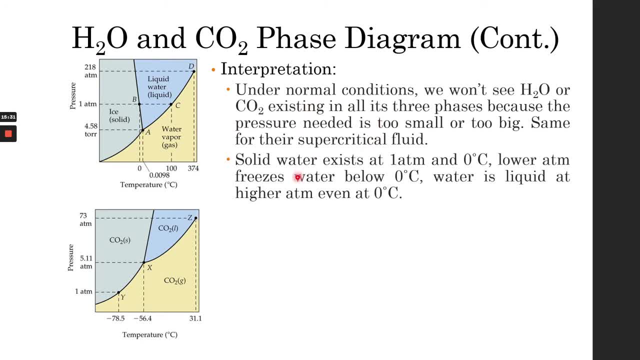 all their three phases. next is that solid water exists at one atmosphere at zero degrees celsius, so that is basically the freezing point of water, so you can create ice when the temperature reaches zero degrees celsius at one atmosphere. but, as you can see, if we actually 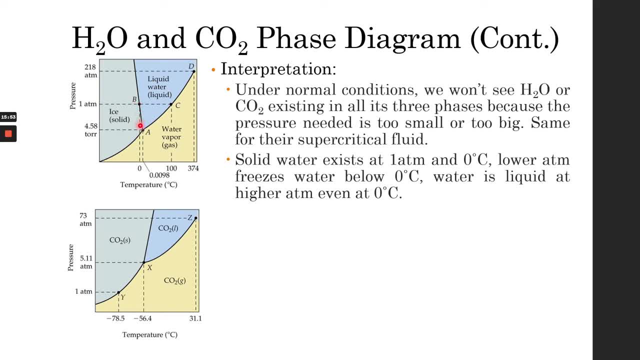 uh, decreases the pressure. so if we go down, when you decrease the pressure, you go higher altitude, so you go on higher, for example on top of a mountain or an airplane. as you can see, if we decrease the temperature even, let's see, we can actually freeze water at a lower atmospheric pressure. we can freeze water below. 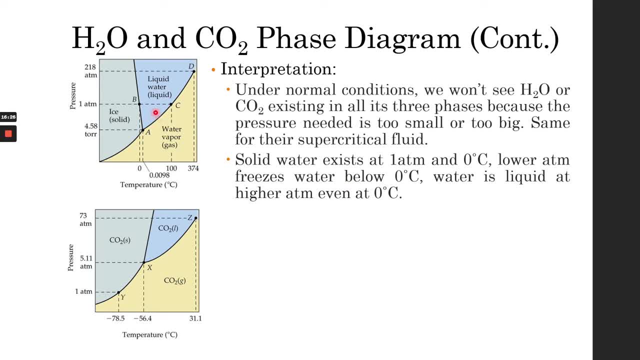 zero degrees celsius and water is liquid at higher. so if we increases the pressure, the, the water or the water is at liquid state even at zero degrees celsius. so liquid vapor ểu at one of these 24, at one atmosphere, at 100 degrees celsius. so you can hear, you see here. so 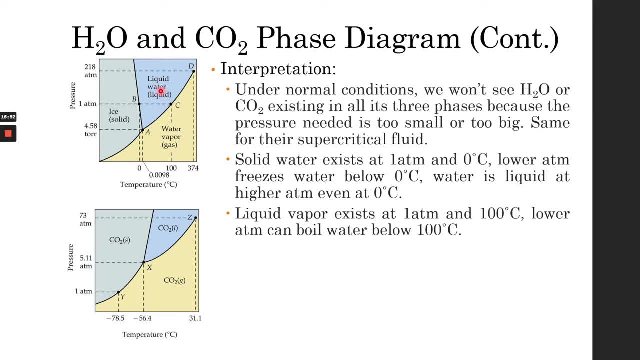 this is the boiling point of water, wherein liquid water turns to gas at 100 degrees celsius. at the same time, if you actually lower the atmospheric pressure, you can boil water below 100 degrees celsius. so if we decrease, for example, one, the atmospheric pressure, you can 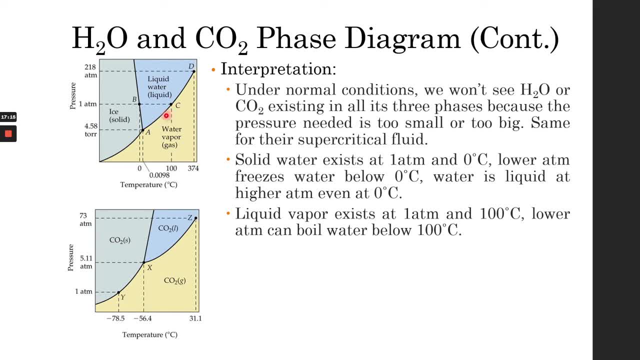 go here so you can actually boil water at lower temperature. okay, the solid and gas phase of co2 exists at one atmosphere and negative 78.5 degrees celsius. so you under, like i said, under normal condition you cannot see solid carbon dioxide, but the same time, you know that we can do it, because 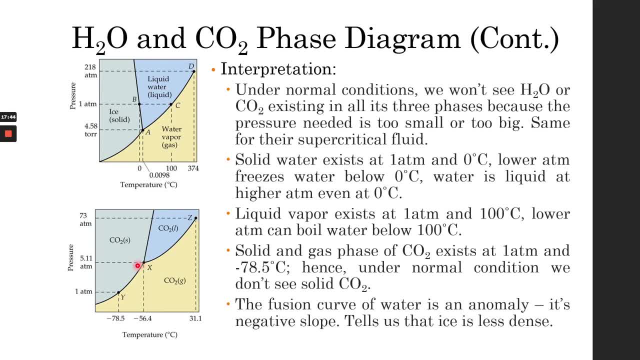 dry ice exists and if you guys look at the fusion curve, so the fusion curve for water is actually at negative slope, while the fusion curve for carbon dioxide is at positive slope. most substances has a fusion curve of positive slope. water is actually an anomaly wherein the fusion curve is actually at 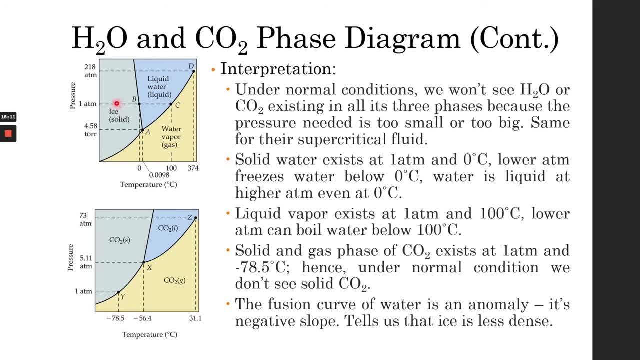 negative slope. this tells us that solid water or ice, is actually less dense than water, which we discussed previously. so even the phase diagram tells us the density of solid water and liquid water and we can see, because it's negative, that solid water is less dense that liquid water, which is opposite for carbon dioxide.